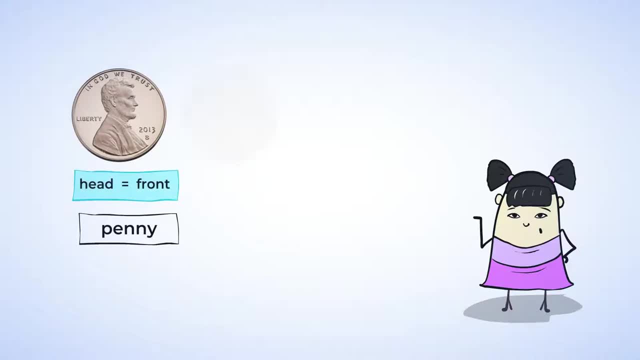 Here is a penny. This is the head of a penny and this is the tail. The head of a coin means the front and the tail of a coin means the back. A penny is worth one cent. We can write one cent with a cents symbol like this, or with a dollar symbol like this. 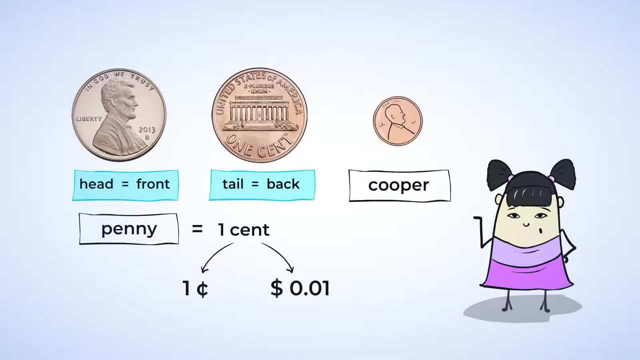 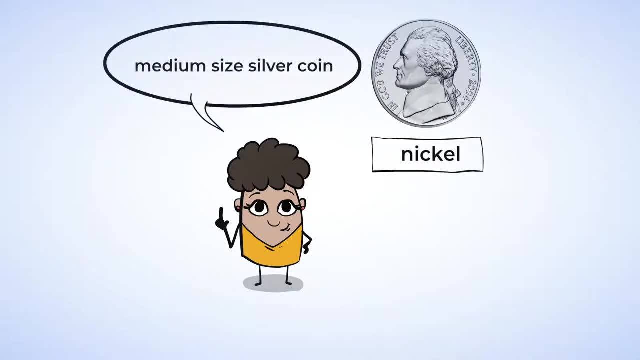 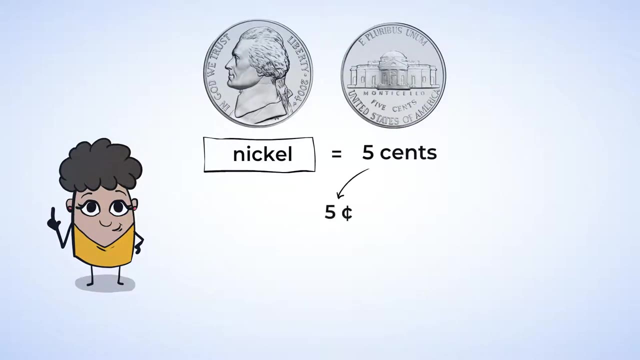 This one is easy to identify because it is copper, not silver, like the other coins. Here is a nickel. It is the medium-sized silver coin and also a little thicker. A nickel is worth five cents and is written using a cents symbol or a dollar symbol. 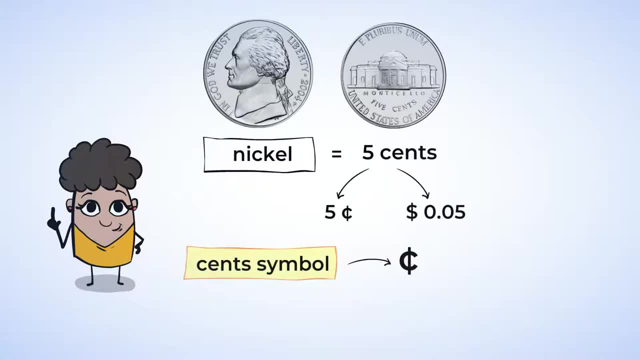 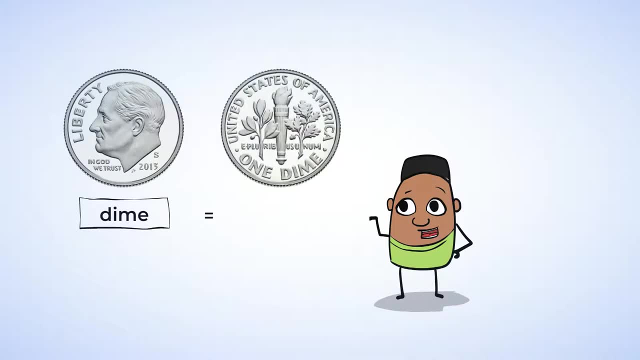 A cents symbol. A cents symbol looks like a C with a line through it. A dollar sign looks like a capital S with a line through it. This is a dime. A dime is worth ten cents and can be written like this: It is the smallest silver coin. 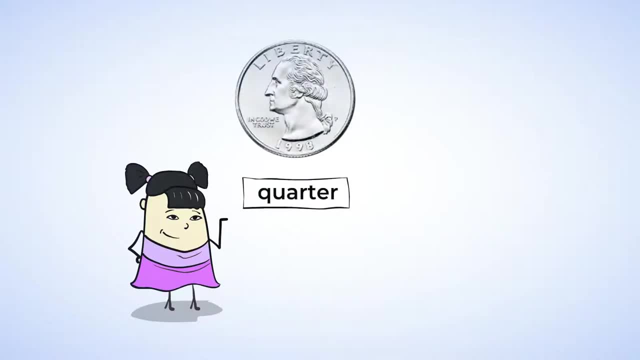 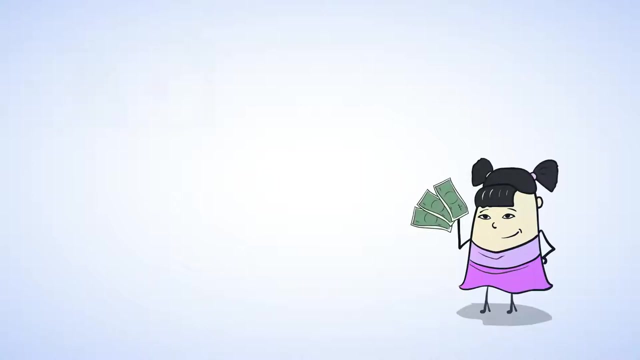 The last type of coin that Sue has is called a quarter. A quarter is worth twenty-five cents. This one is the largest silver coin. I like the eagle that it usually has on the back. Sue also has some dollar bills. This is the front and the back of a dollar bill. 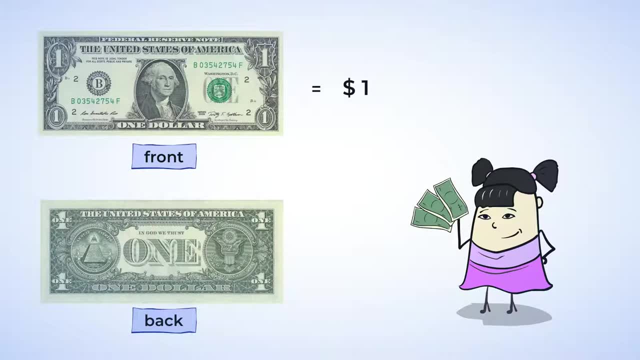 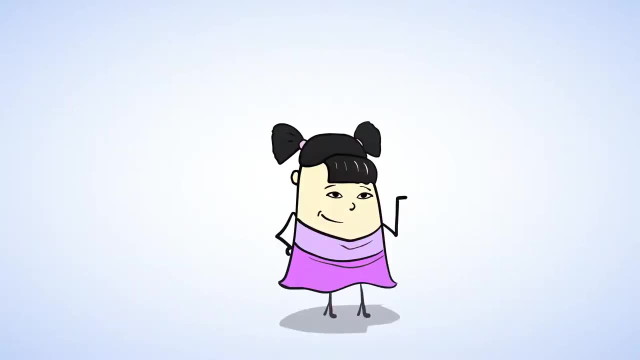 A dollar bill is worth one dollar and can be written only with a dollar sign like this: Now we are going to see some different combinations of coins. If you want to go get some coins of your own to use, go ahead and pause this video to get some. 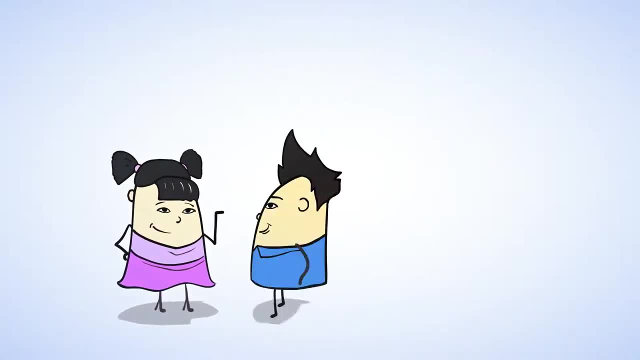 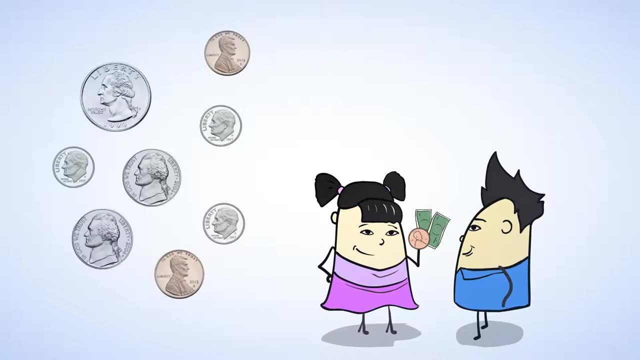 We'll wait. Sue promised her little brother she would give him some money for gum at the store. Here are some coins. Here are the coins she gave him. One way to count up all the coins is to find the total value of each coin type and add them. 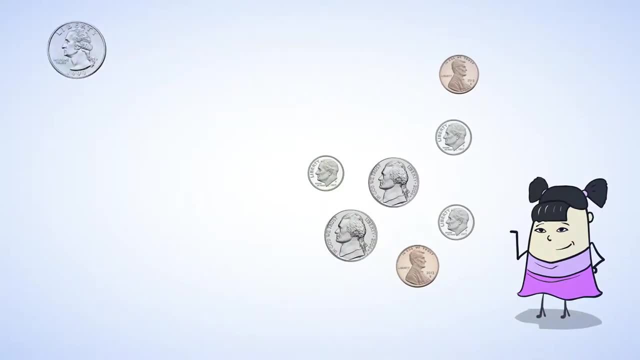 Let's try that. To start, there is one quarter, which is twenty-five cents. Next count the dimes. There are three dimes. Since a dime is worth ten cents, we can skip count by tens to find out how much the three. 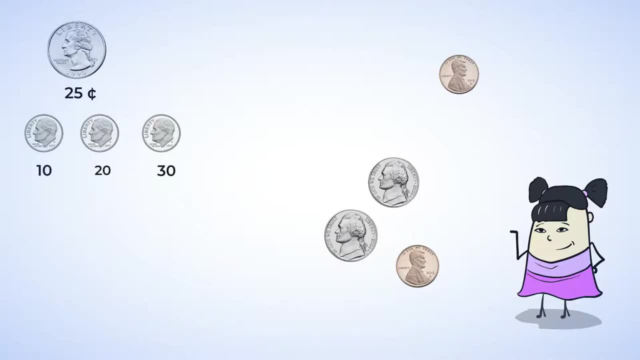 dimes are worth Ten, twenty thirty. These dimes are worth thirty cents altogether. Let's count the nickels. now There are two nickels. Each nickel is worth five cents, so two nickels are worth ten cents, since five plus five. 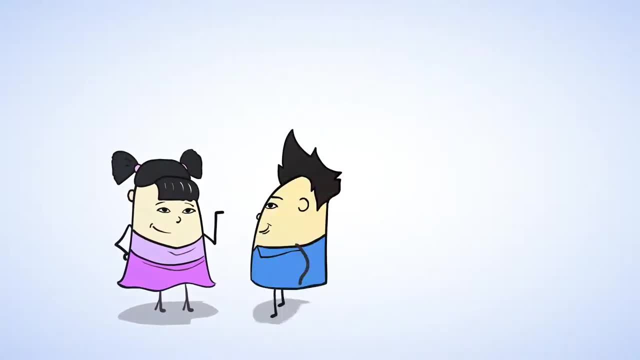 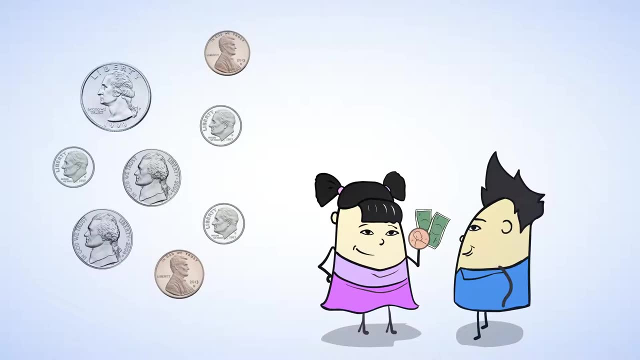 We'll wait. Sue promised her little brother she would give him some money for gum at the store. Here are the coins she gave him. One way to count up all the coins is to find the total value of each coin type and add them. 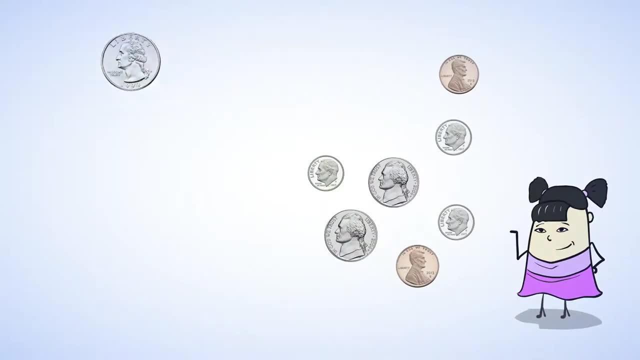 Let's try that. To start, there is one quarter, which is twenty-five cents. Next count the dimes. There are three dimes. Since a dime is worth ten cents, we can skip count by tens to find out how much the three dimes are worth. 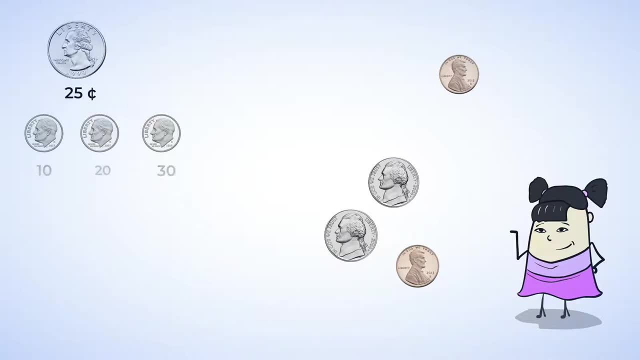 Ten, twenty, thirty. These dimes are worth thirty cents. Here are the coins she gave him. They are worth thirty cents altogether. Let's count the nickels. now There are two nickels. Each nickel is worth five cents, so two nickels are worth ten cents, since five plus five. 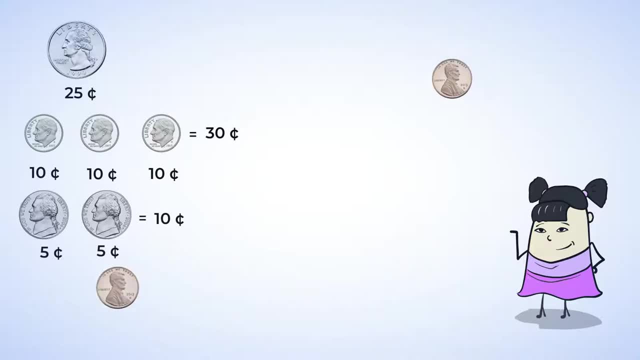 equals ten. Lastly, there are two pennies. Each penny is worth one cent, so two pennies are worth two cents. We have twenty-five cents, thirty cents, ten cents and two cents. Let's add up these amounts to find the total value. 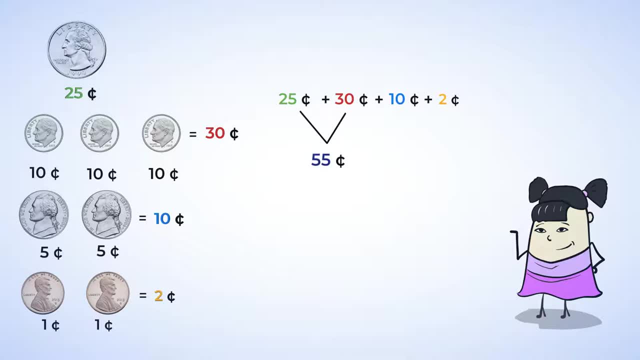 Twenty-five plus thirty is fifty-five. We can find that by skip counting up by tens. Twenty-five, thirty-five, forty-five, fifty-five, Fifty-five plus ten is sixty-five, And sixty-five plus two is sixty-seven. Sue gave her brother sixty-seven cents. 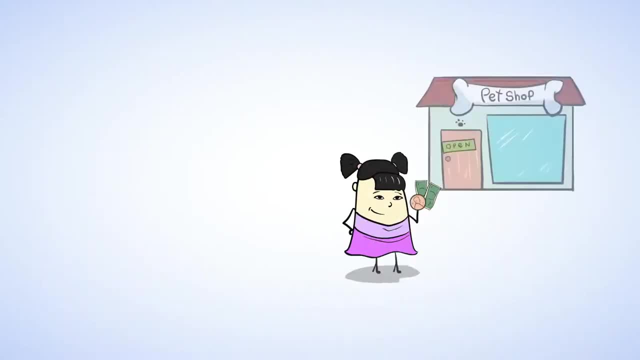 Great work. Now Sue is taking some money for her trip to the pet store. Here is what she is taking. Let's figure out how much money Sue is taking. Here is what she is taking. Let's figure out how much money Sue is taking. 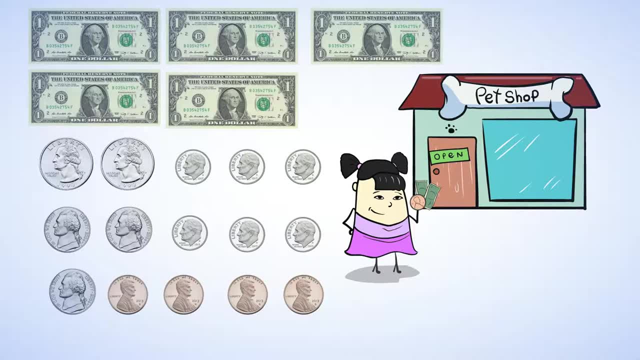 Here is what she is taking. Let's figure out how much money Sue is taking. She has five dollar bills, That is five dollars to start. Now. let's set those aside. as we count up all the coins, Often times it is easiest to start with the coins that have the largest value. 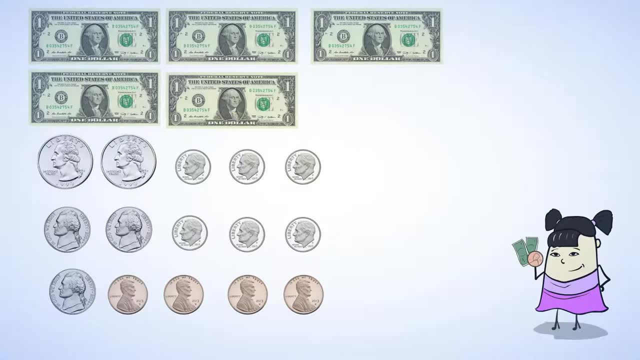 That's the quarter, so let's start there. There are two quarters. Each quarter is worth twenty-five cents, so that is fifty cents. since twenty-five plus twenty-five is fifty, The next largest value is the dime. That is ten cents each, and there are six of them. 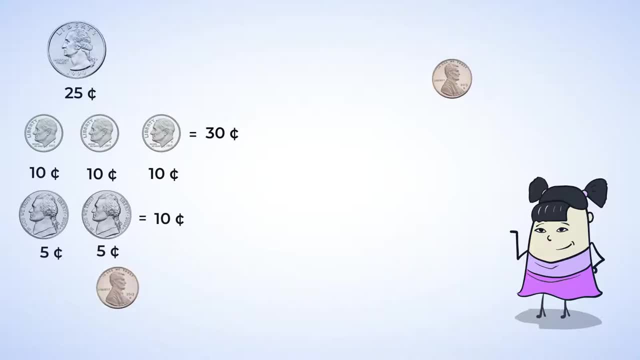 equals ten. Lastly, there are two pennies. Each penny is worth one cent, so two pennies are worth two cents. We have twenty-five cents, thirty cents, ten cents and two cents. Let's add up these amounts to find the total value. 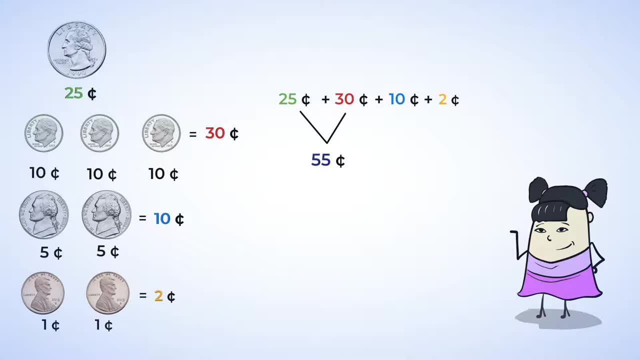 Twenty-five, Twenty-five plus thirty is fifty-five. We can find that by skip counting up by tens, Twenty-five, thirty-five, forty-five, fifty-five, Fifty-five plus ten is sixty-five, And sixty-five plus two is sixty-seven. 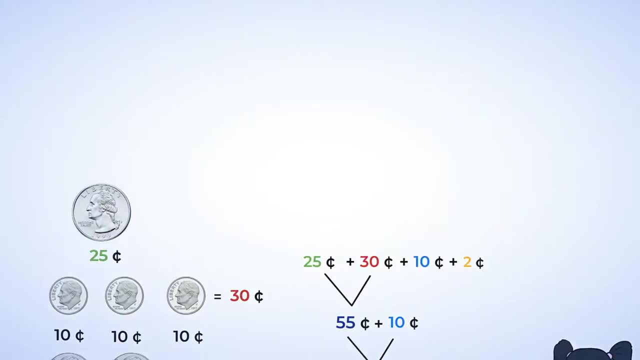 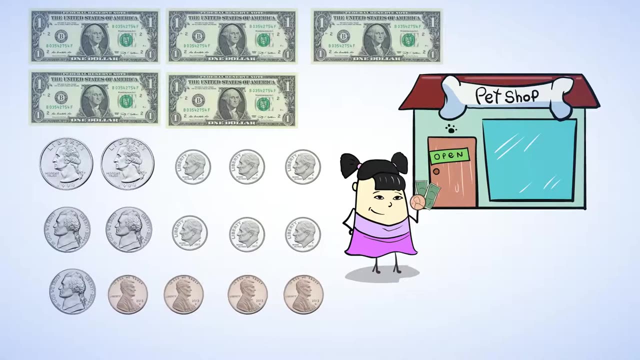 Sue gave her brother sixty-seven cents. Great work. Now Sue is taking some money for her trip to the pet store. Here is what she is taking. Let's figure out how much money Sue is taking. She has five dollar bills. That is five dollars to start. 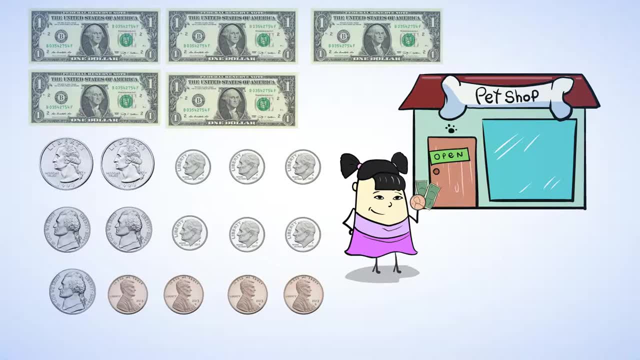 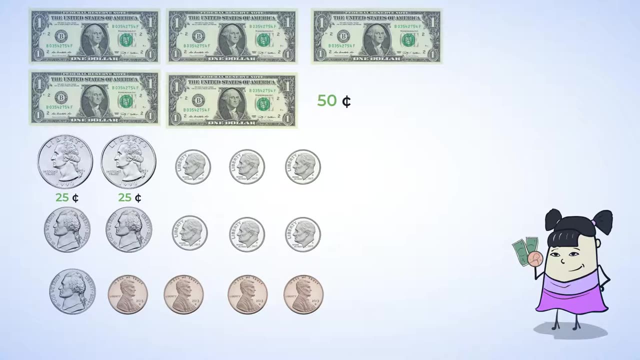 Now let's set those aside. as we count up all the coins, Often times it is easiest to start with the coins that have the largest value. That's the quarter, so let's start there. There are two quarters. Each quarter is worth twenty-five cents, so that is fifty cents since twenty-five plus. 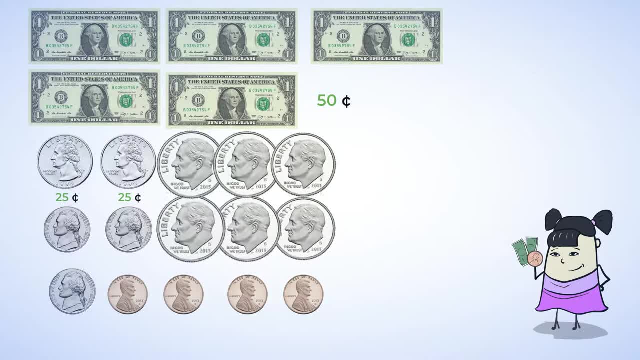 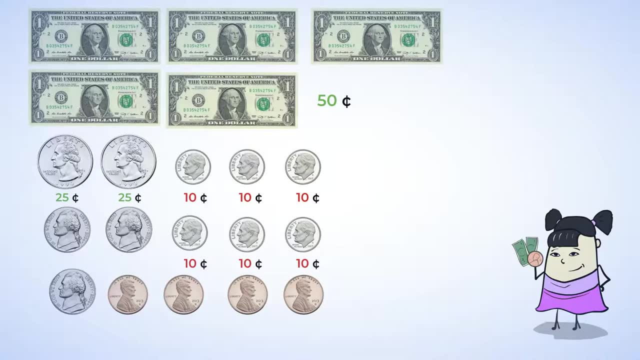 twenty-five is fifty. The next largest value is the dime. That is ten cents each, And there are six of them. Let's skip count by tens to find the total value of the dimes. Ten, twenty, thirty, forty, fifty, sixty. 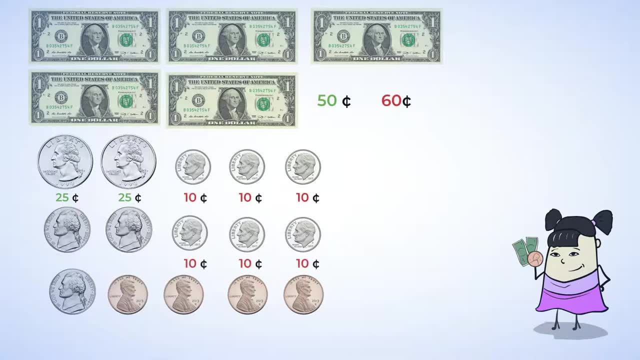 These dimes are worth sixty cents. Then there are the nickels. There are three nickels, so skip count by fives to find the value of the nickels. Five, ten, fifteen: These nickels are worth fifteen cents. Finally, there are four pennies. 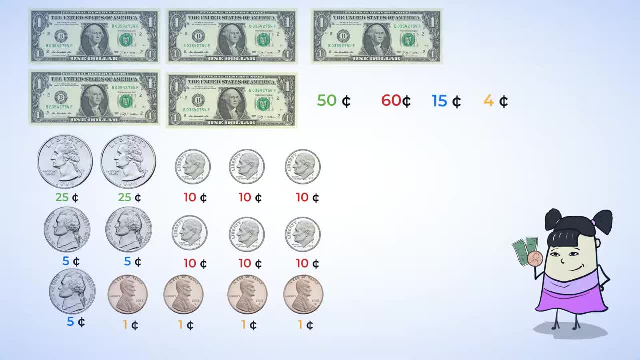 Since each penny is worth one cent, that is four cents altogether. Let's add up the value of all the coins. First we have fifty cents and sixty cents. Together, that makes one hundred ten cents. Then add fifteen cents to get one hundred twenty-five cents. 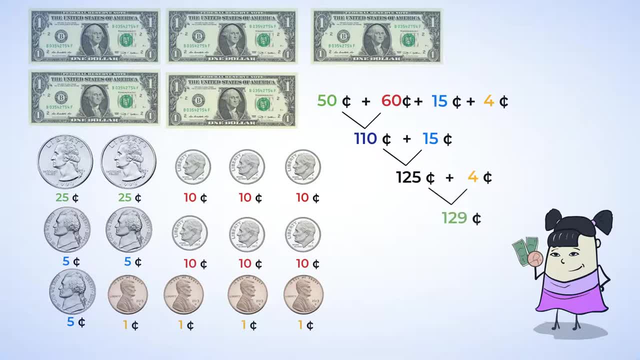 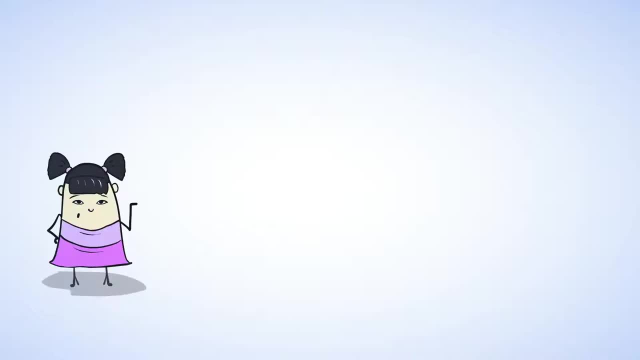 Finally add four cents to get one hundred twenty-nine cents. That's a lot of cents. You probably don't hear many people talk about more than one hundred cents at a time. That's because once you have reached one hundred cents, you have a whole dollar. 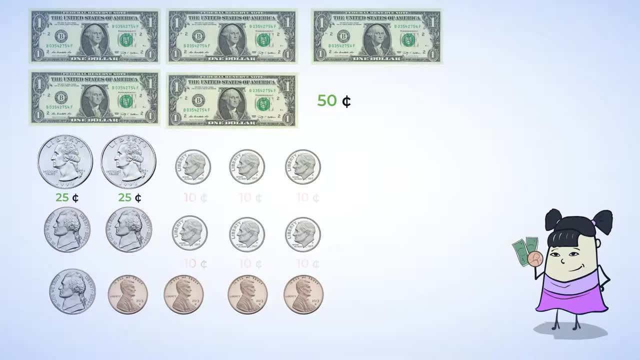 Let's skip, count by tens to find the total value of the dimes. Ten, twenty, thirty, forty, fifty, sixty. These dimes are worth sixty cents. Then there are the nickels. There are three nickels, so skip, count by fives to find the value of the nickels. 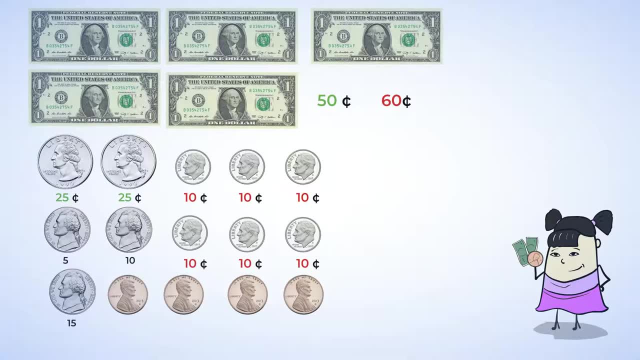 Five, ten, fifteen. These nickels are worth fifteen cents. Finally, there are four pennies. Since each penny is worth one cent, that is four cents altogether. Let's add up the value of all the coins. First, we have fifty cents and sixty cents. 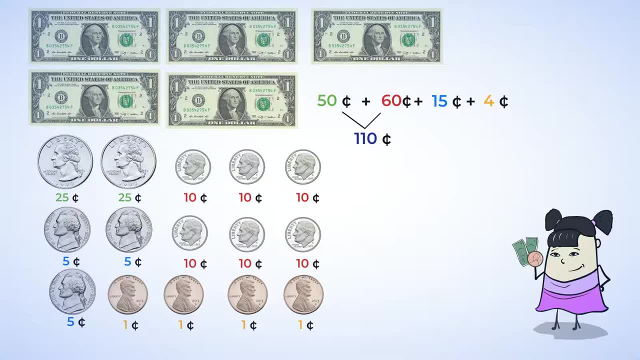 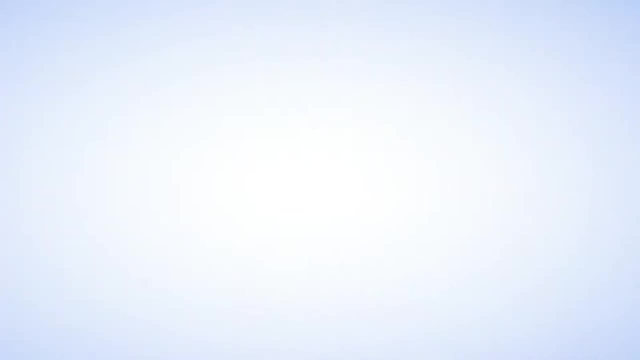 Together that makes one hundred ten cents. Then add fifteen cents to get one hundred twenty-five cents. Finally, add four cents to get one hundred twenty-nine cents. That's a lot of cents. You probably don't hear many people talk about more than one hundred cents at a time. 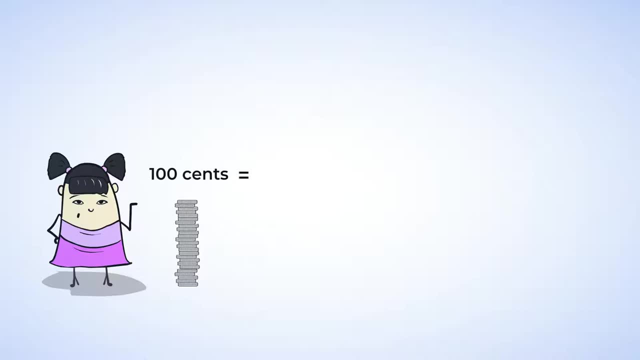 That's because once you have reached one hundred cents you have a whole dollar. One dollar equals one hundred cents. That's a lot of cents. So we can subtract one hundred from one hundred twenty-nine and add that dollar of coins to our five dollar bills. 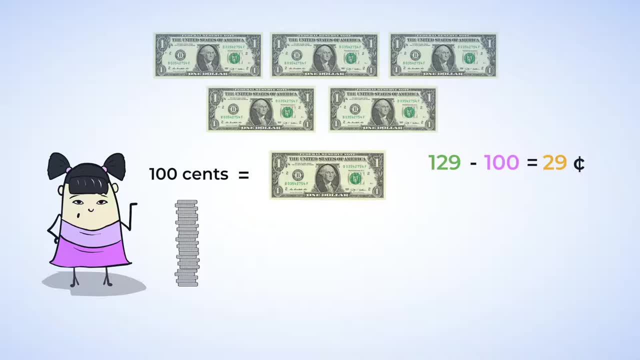 That leaves us with twenty-nine cents. So we have the five dollars from the bills. That's a lot of cents. One dollar from the coins and twenty-nine cents from the coins. Together that makes six dollars and twenty-nine cents. We can write that like this: 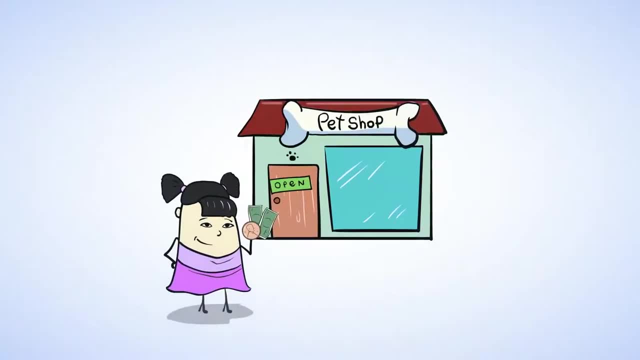 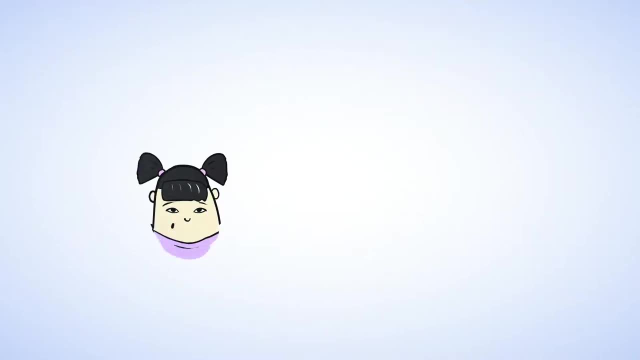 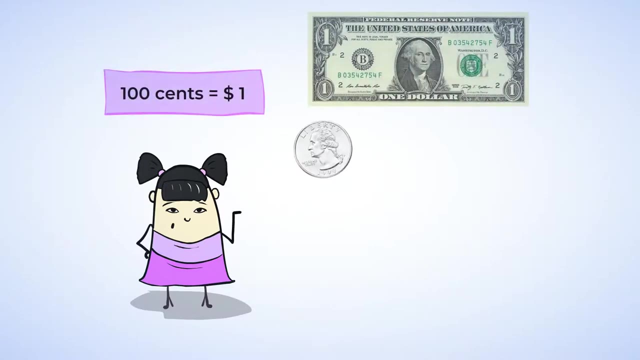 Six dollars and twenty-nine cents. So Sue is taking six dollars and twenty-nine cents to the pet store. Great work. You have learned about the value of different coins and the dollar bill. You know that a dollar bill is worth one dollar. A quarter is worth twenty-five cents. 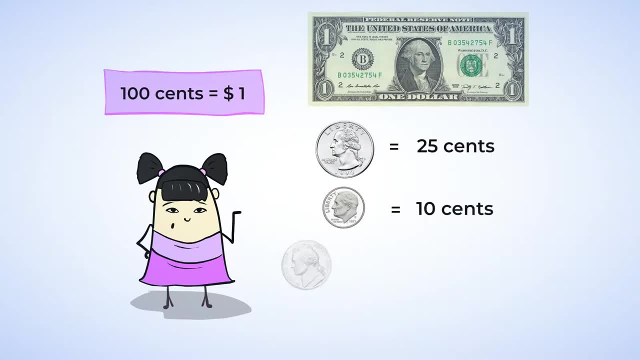 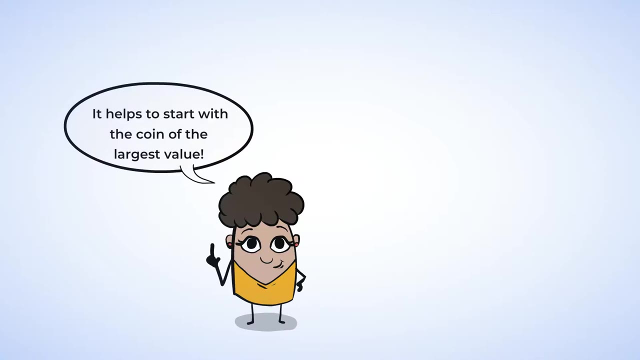 A dime is worth ten cents, a nickel is worth five cents and a penny is worth one cent. You have learned strategies for counting up coins of different values. Often it helps to start with a coin of the largest value. You can count the value of each coin type and then add them all together.